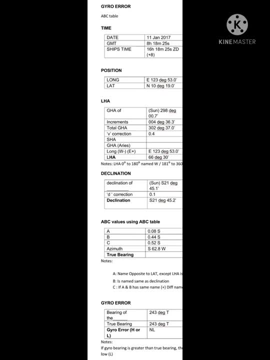 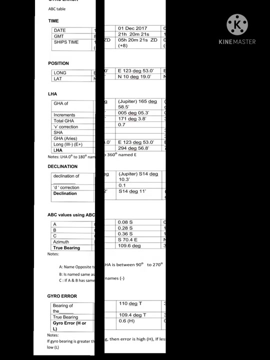 And the gyro error bearing of the 243 degrees true. true bearing is 243.. degrees true, so on. so let's proceed to the next, which is that Jupiter. so date is 1 December 1 2017. JMT is 21 hours 20 minutes 21 seconds, so ships time is 0: 5. 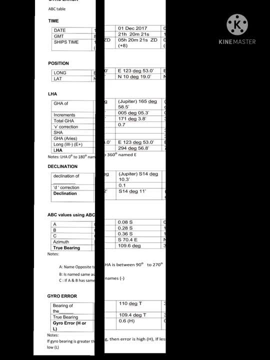 hours 20 minutes 21 seconds. zone description is plus 8, so our position of longitude is east, 21 degrees 53 minutes, and latitude is nor at North, 10 degrees 19 minutes. so the H a of Jupiter is 165 degrees fifty eight point five minutes, and then increments is five degrees and zero. 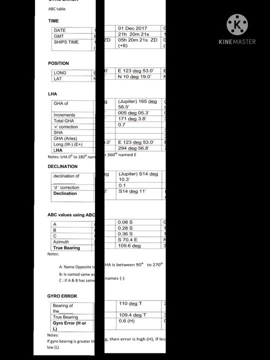 point five minutes and then increments is five degrees and zero point five minutes and then five minutes and then increments is five degrees and then increments is five degrees and then H? a is one hundred seventy one degrees and three point eight minutes and- V correction- zero point seven. so we don't have the SH a and GHA of Aries in here, so our longitude will be East. 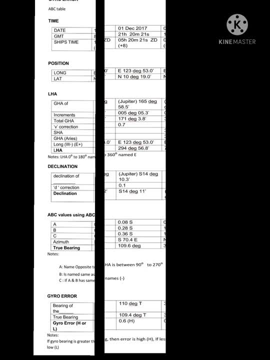 21, 23 degrees, 53 minutes, and the LHA will be two hundred ninety four degrees fifty, 56.8 minutes. declination of Jupiter is south 14 degrees, 10.3 minutes, and D correction will be 0.1. you just have to add. so south 14 degrees and 11. 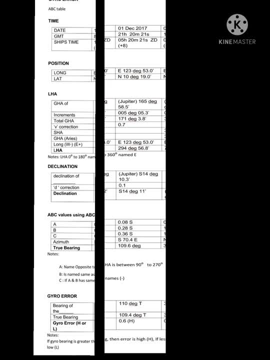 minutes. so our ABC will be, our a will be 0.08 South and B will be 0.28 South. just have to add it. so come up with: and RCU will be 0.36 South and the Azimut will be South 70.4 East. so our true bearing here is 109.6 degrees and a. 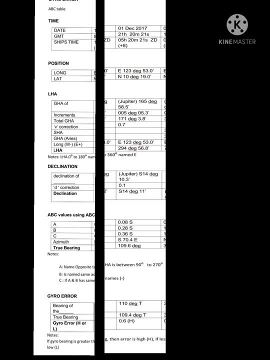 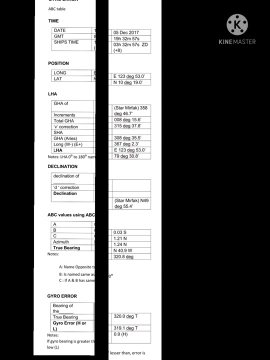 bearing of the Jupiter is 110 degrees true, and true bearing will be one hundred nine point four degrees true, and our gyro error will be 0.6 high. so let's proceed to star merfolk. date will be 05 december 2017. jmt will be 19 hours 32 minutes 57 seconds. the ship's time will be: 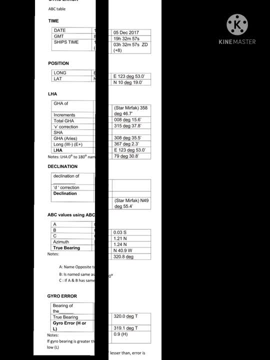 03 hours 32 minutes 56, 57 seconds, and our zone description will be plus eight. so position of longitude is 130 degrees 53 minutes east and our latitude will be 10 degrees 19 minutes north, and lha of starmer, jha of star merfolk is 358 degrees 46.7 minutes. increments will be: 008 degrees, 15.6 minutes, and a total jha of 315 degrees, 37 minute, 0.8 minutes. so we don't have a correction and our sha will be 308 degrees, 35.5 minutes and our jha of aries will be 367 degrees. 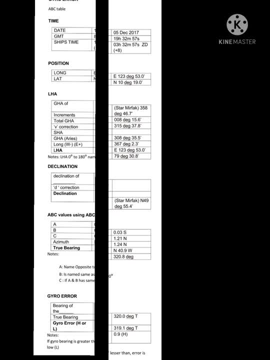 2.3 minutes and our longitude will be 0.6 long. uh, so so a longer longitude will be 123 degrees 53.0 minutes. east lha will be 79 degrees 30.8 minutes, and declination of star merfolk is known in the correction, so our declination will be: 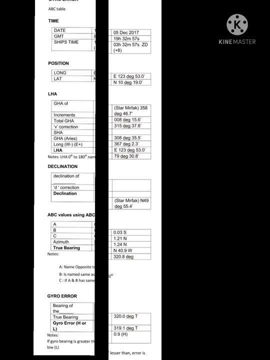 49 degrees, 55.4 north. so abc volume use will be: uh, the a will be 0.03 south and b will be 1.21 north. we just have to subtract it because this opposite, so our c will be one point, i mean add. so our c will be 1.24 north. azimuth will be: 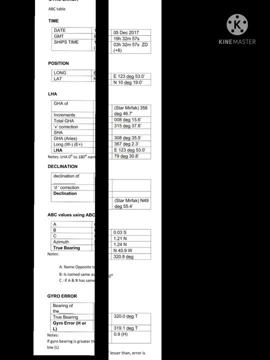 north, 40.9 west natural bearing will be true to 320 point 8 degrees. now general error will be: uh, the bearing of the star merfolk is 20 320 degrees true, and our true bearing will be g- 19.1 degrees true, and our gyro error will be 0.9 high. so that's all, thank you.